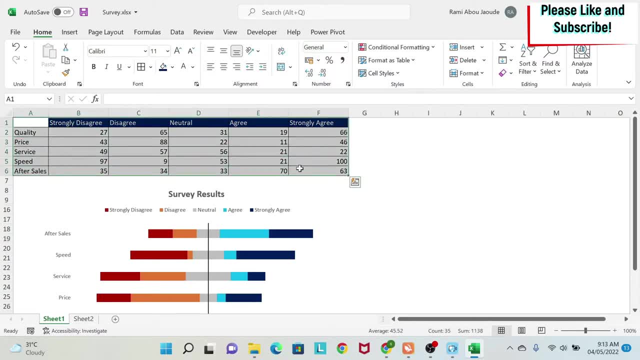 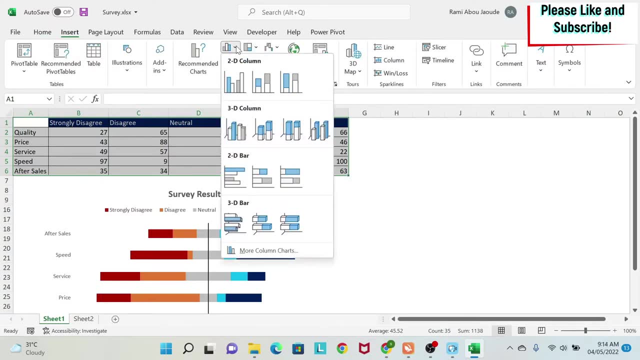 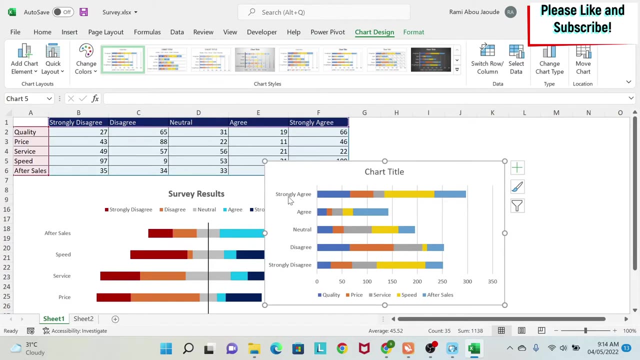 I have a few metrics. A lot of time, what we would do in Excel is just select this and go to insert and then under insert you have here some 2d bars and then, if you select this, you can get this kind of charts. if you see, here I have the. 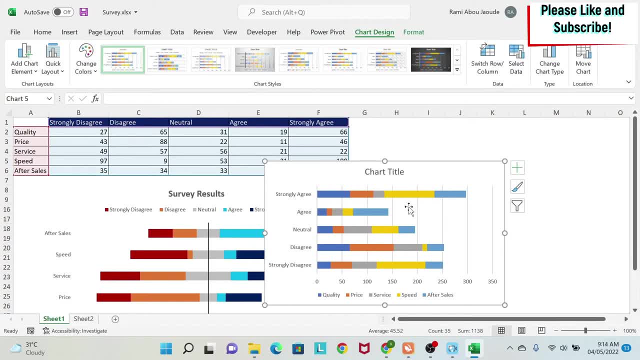 strongly agree, and so on. here I don't want them. I want actually the opposite. so I right-click, select data, switch row and column, and I get something like this: if I look at this, I have the number of people who are in each category for each type of chart. 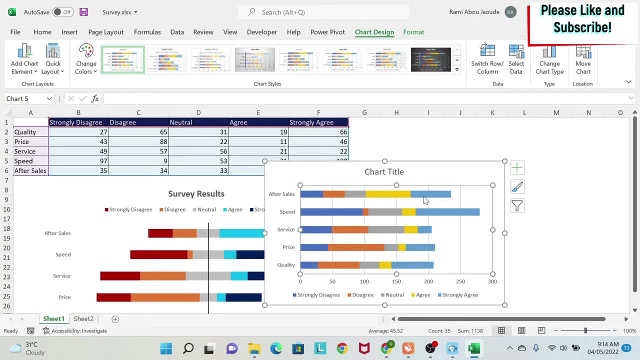 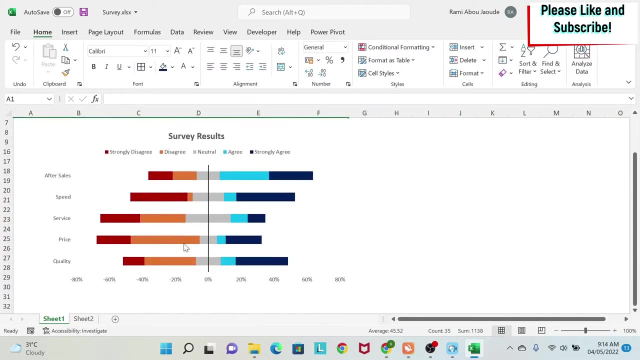 The problem is, if I show this in a meeting, it is very hard to make anything of it and understand really what has happened, right, what should be the action course here. it's very hard to know, so instead we can do something like this, which looks much neater and shows you the percentage of people that are on: 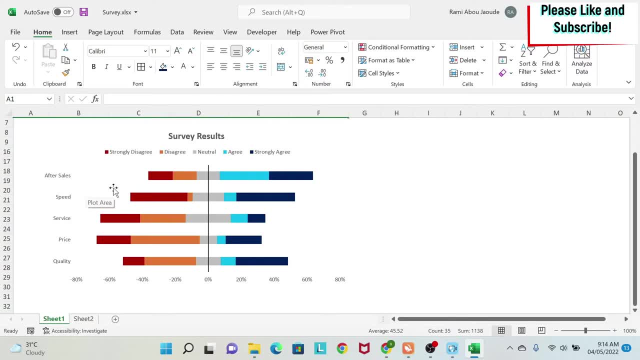 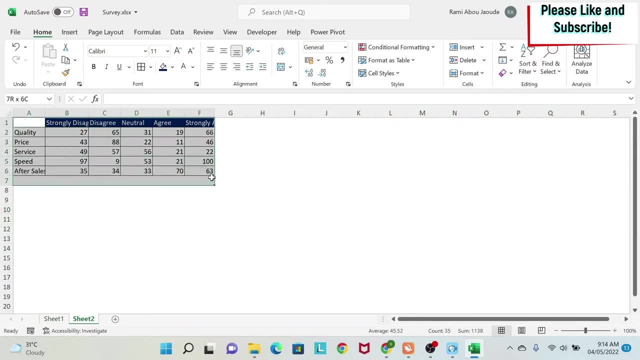 the positive side and the percentage of people on the negative side. So let's start and let's do it together. First step: here you have the data. so I'm going to copy paste the data, so I'm going to select it- ctrl C- I go here, I do paste, paste, special paste link. I'm going to 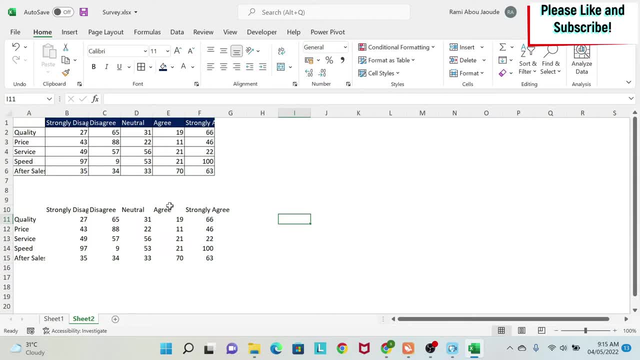 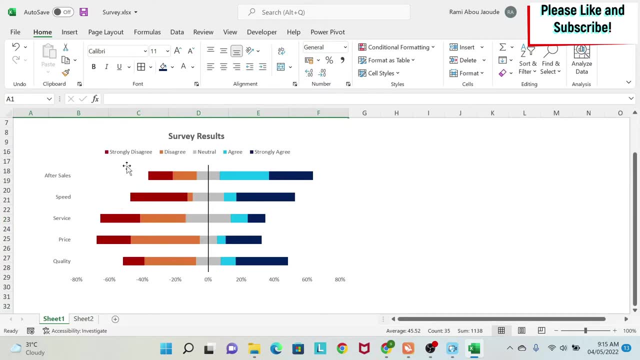 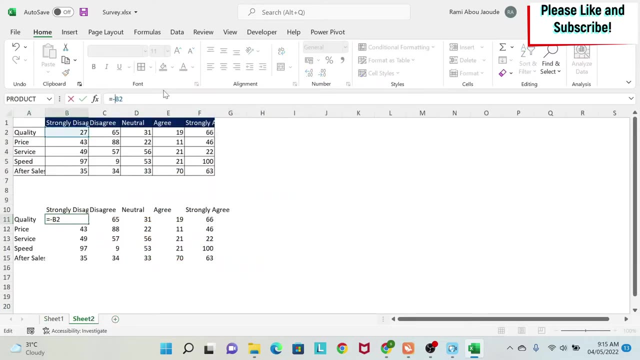 remove the zero and then I'm going to play my first trick. if you see, here I have positive values and negative values. what does it mean? it means that everything that is on this side- I have to put a minus for it- so strongly disagree. we're gonna put the minus in front of the b2 and here we're gonna put. 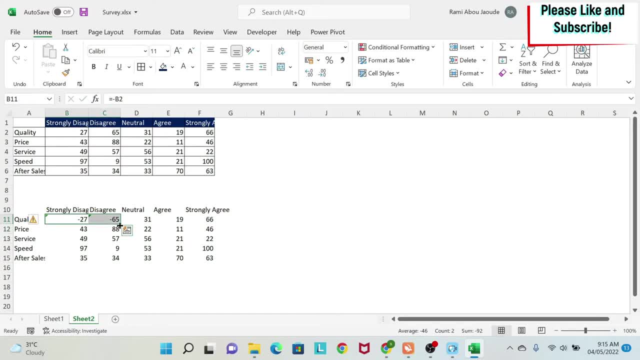 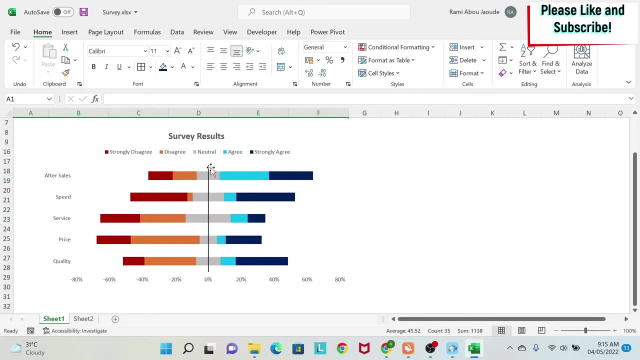 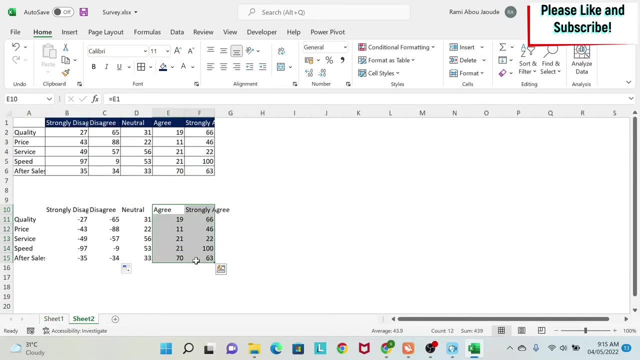 a minus, then we can drag those two formulas down and then the trick is completed. second trick: if you see here the neutral, part of it is on the negative and part of it is on the positive right. so what will I do? I'm just gonna select this, move it like this, as you can see. select another neutral. 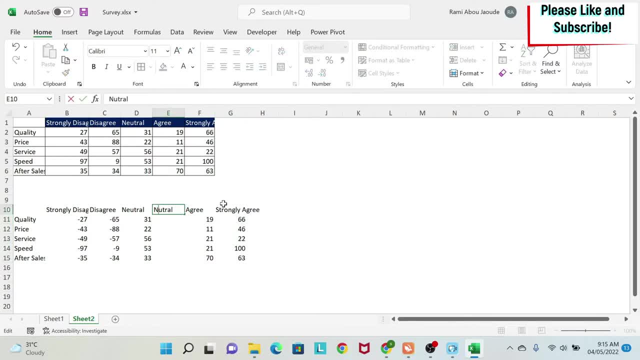 column, then we're gonna divide this neutral into two. so we're gonna do this divided by two and we're gonna drag it down by double clicking here and here. we're gonna do this divided by two and we put the minus because we want it on the. 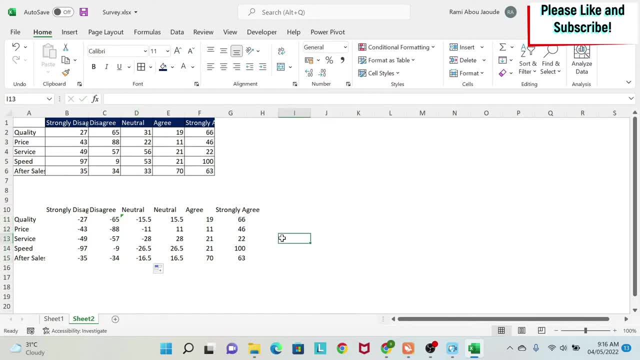 other side, same thing. we're gonna drag it. there you go. if you see, here I still have my 31 value, but half of it is on this side, half of it is on the other side. now we're gonna try to insert a chart and I'm gonna show you the problem. 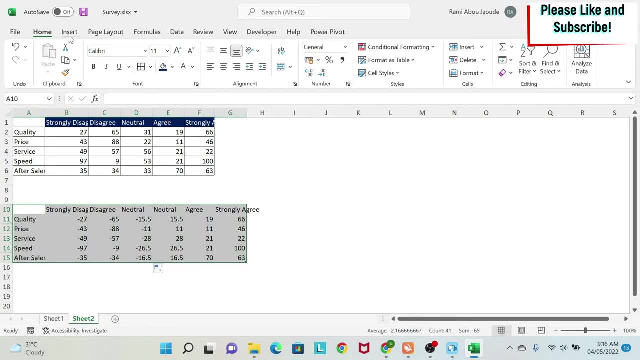 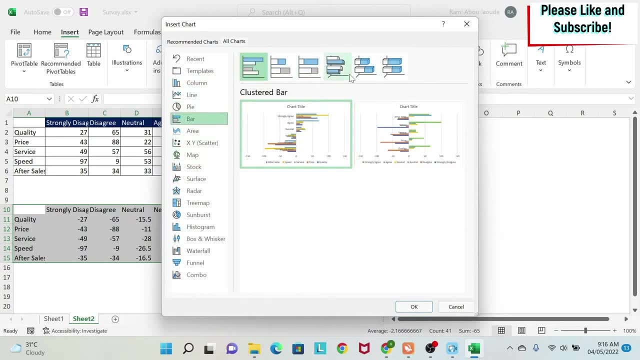 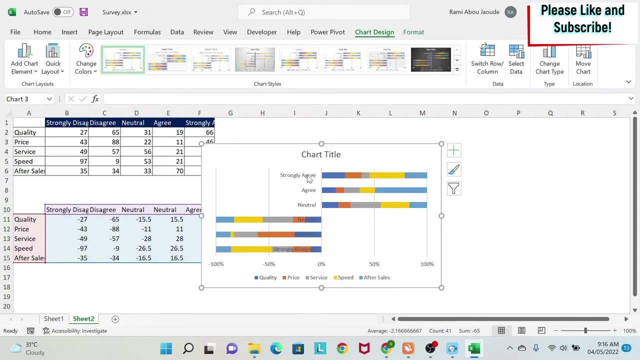 that you're gonna encounter. so let's select the data, do insert, we click here, we go to all charts and then we can select bars. we have this one, for example, and we can say: ok, if you see, here again I have the strongly agree, etc. on the 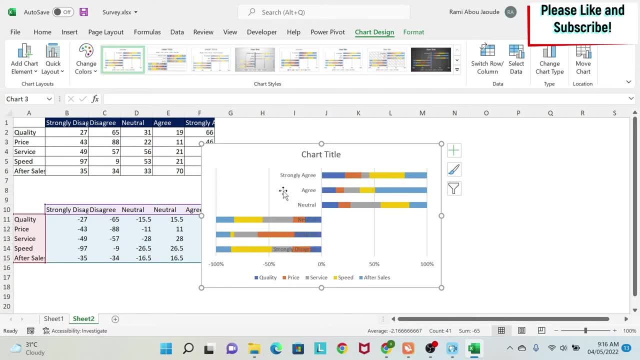 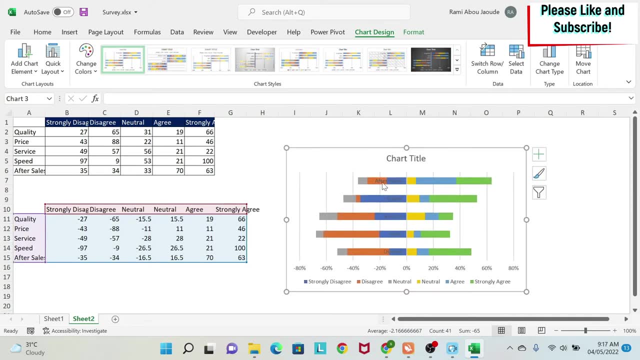 axis. I want the opposite. I want them as a legend. so I right-click, select the data, switch row and column, and we have this. so if you see, here, the labels are coming on the graph and I don't want this. so how to fix this? I'm gonna click. 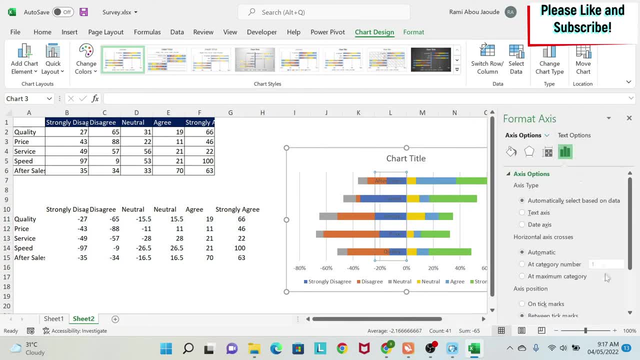 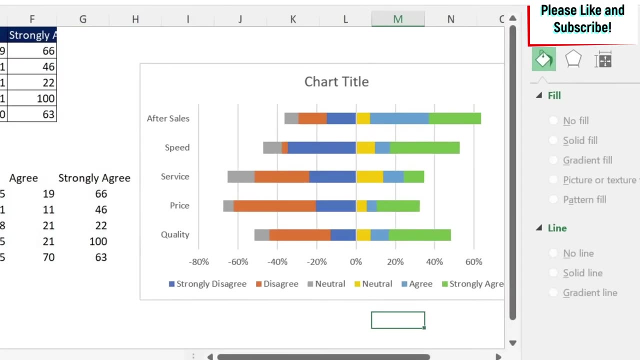 on them, right click format axis. I go here on the bottom I have label, and then here I have label position. you have to select low. when you select low, they are here. so everything is good. the problem I'm facing if I close this is that if you see here, strongly, disagree is coming here. 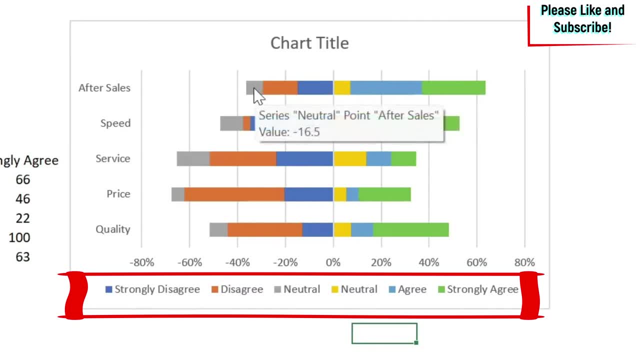 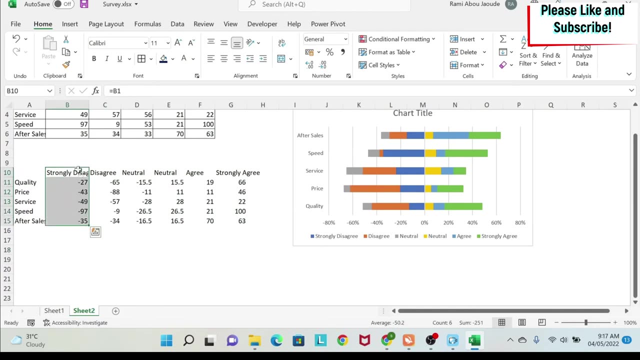 disagree is here and neutral is here. but what I want? I want the opposite. I want neutral here, disagree in the second position and strongly disagree here. so what I'm gonna do is just switch them. so here we go, we just take them. we put them here, we take neutral. 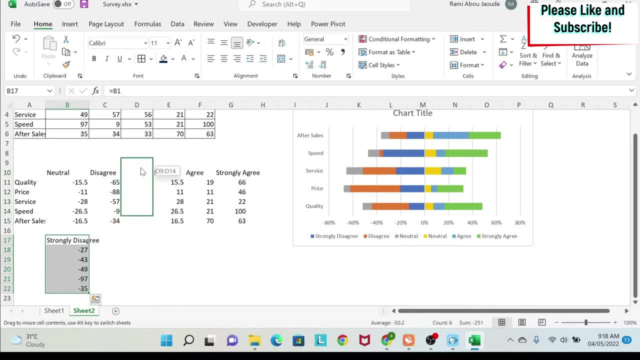 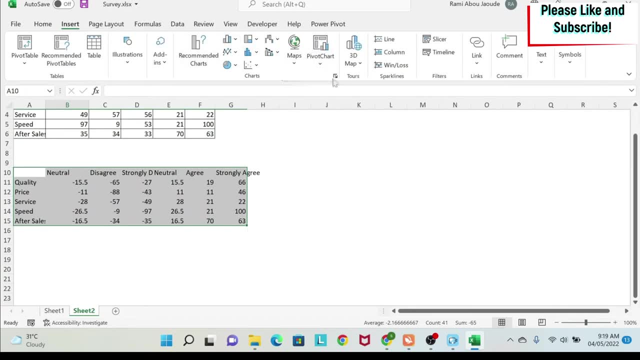 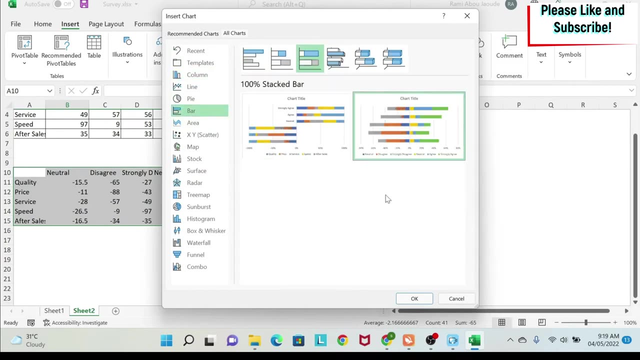 we put them here and then we put this one back here. so let's remove the chart and put it again. so we go here and we do insert. we select the right chart. all chart bars select this. this one that I selected is here. we do this, we click on. 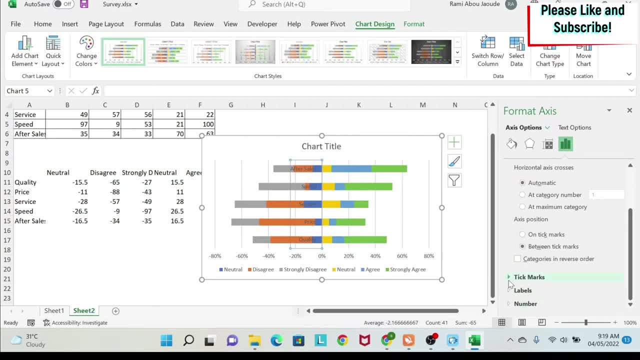 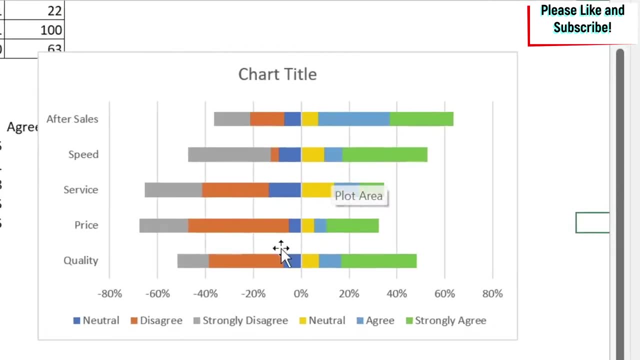 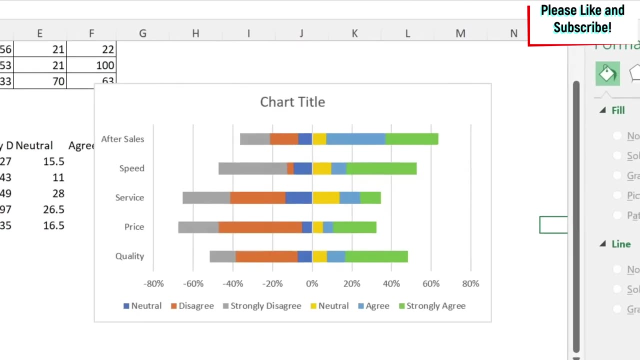 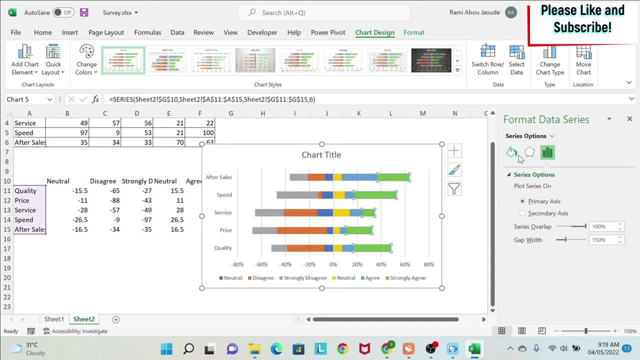 this right click format: access labels low, and then we see that we have the. then, if you see, i have strongly disagree here now. disagree is here and neutral is here. next, we need to take care of the colors. so, for the colors, you click on this one, you go to the bucket and you 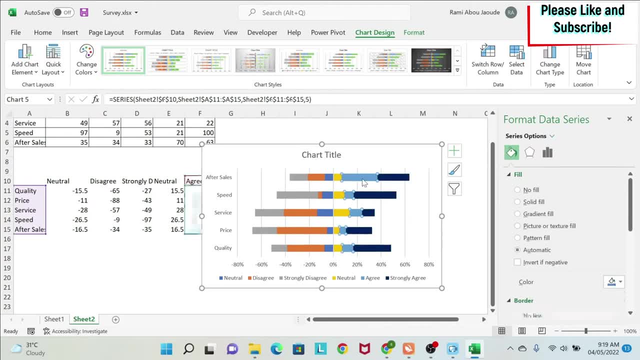 select the color that you like. i personally like this one. here i'm gonna do the same. i'm gonna select this blue. here i need a gray, so i'm going to select this gray. same for this one. this is gray. then here we have orange, which is fine, and here i'm going to select some kind of red. 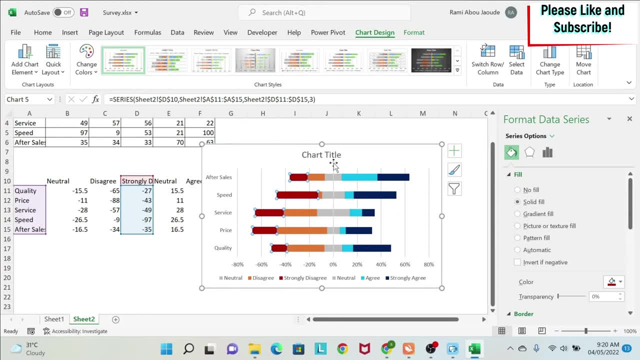 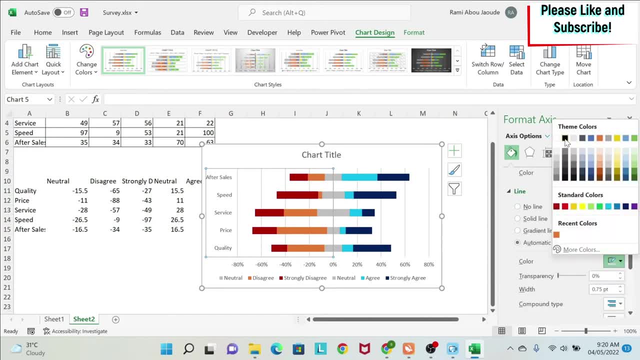 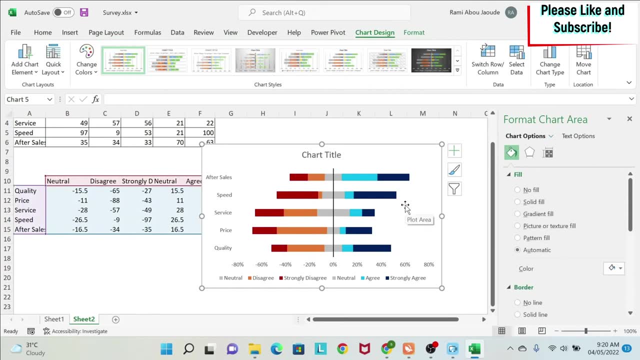 the color of the line here, so i'm gonna make it black. so we have the color of the line. we click on those grid lines one time we press delete they are gone and then we need to play with the legend. so if you see, here i have a second neutral that i don't want. you see, i have neutral and neutral. 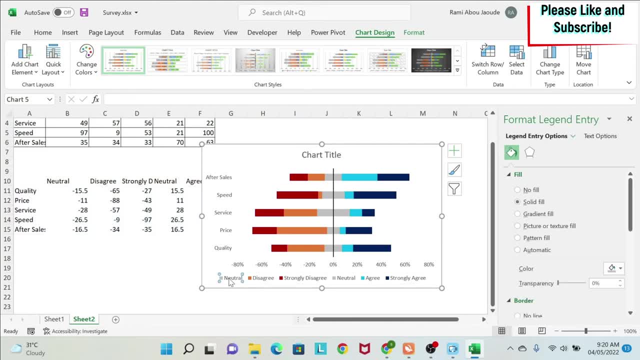 so i can click one time, two time, on neutral press delete. it's gone. the last problem i'm facing is that if you see i have disagree, then strongly disagree on the legend and i want the opposite. so how to fix this? well, there is a trick. i'm going. 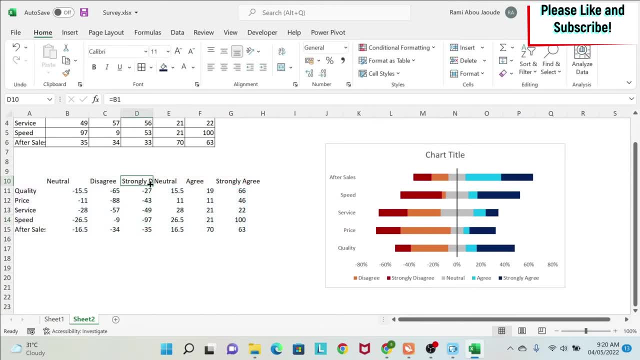 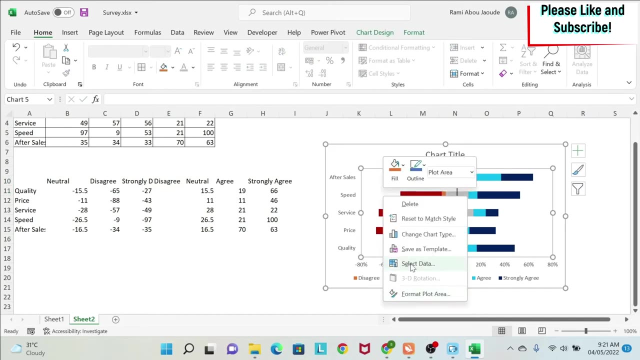 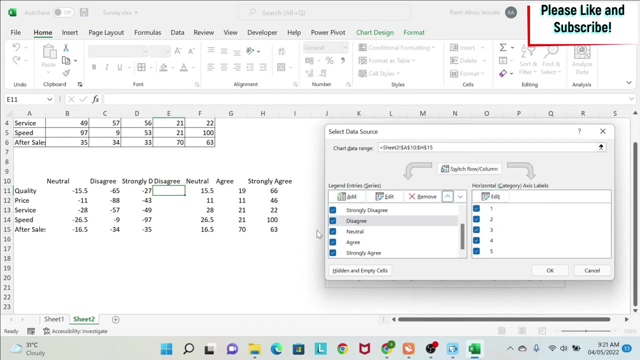 to show you. so what we're gonna do now is we're gonna move this here, then we're gonna do another disagree here with no data and i'm gonna add this series to the chart select. then i do add series name disagree series name values. i take the empty values, i say okay, and then i can move it up. so, for example, if i put it: